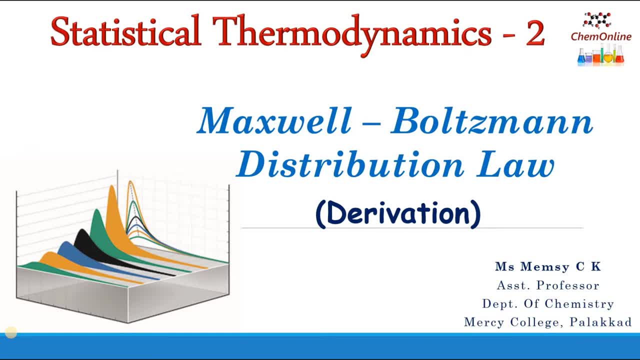 Dear students, in the previous class we had a general introduction to statistical thermodynamics. In this video we will have a discussion on Maxwell-Boltzmann statistics. The Maxwell-Boltzmann distribution concerns the distribution of an amount of energy between identical but distinguishable particles. 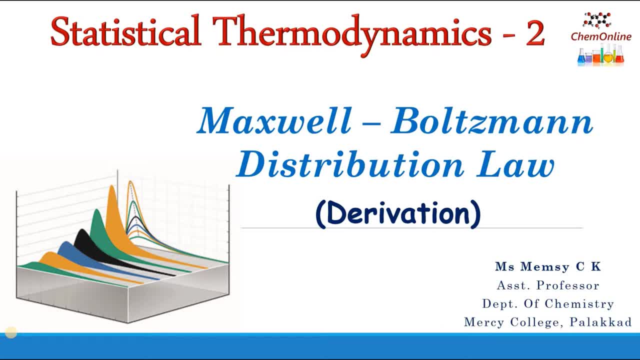 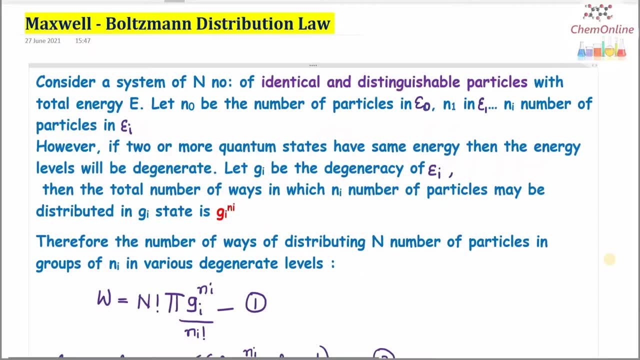 Thus it represents the probability for the distribution of the states in a system having different energies. Today, we will have a discussion on Maxwell-Boltzmann distribution law. We know that there are three types of statistics in statistics: One is Maxwell-Boltzmann, second is Bose-Einstein, third is Fermi-Dirac. 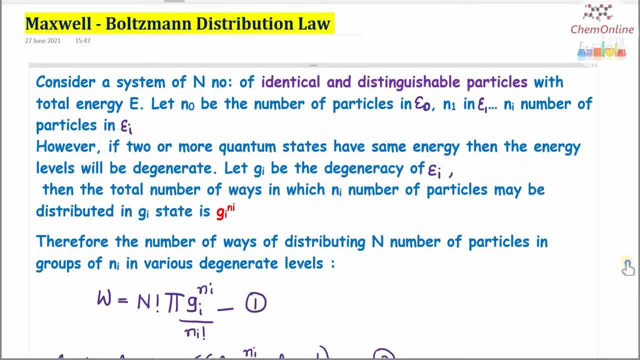 Today we are going to see the first type of statistics, Maxwell-Boltzmann statistics. I will have Maxwell-Boltzmann distribution law derived from this Suppose: we have n number of identical and distinguishable particles with total energy E. So total number of particles is n and total energy is E. 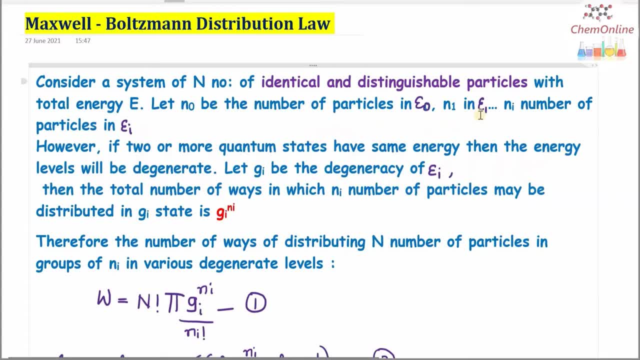 Let n0 be the number of particles in epsilon 0,. n1 in epsilon 1, ni number of particles in epsilon i. Now, if we are considering the degeneracy of the energy levels, let gi be the degeneracy of epsilon i. 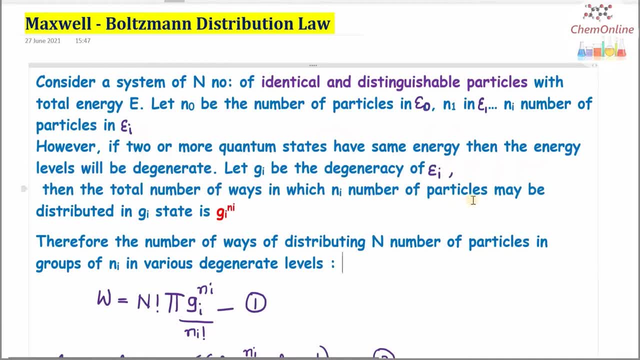 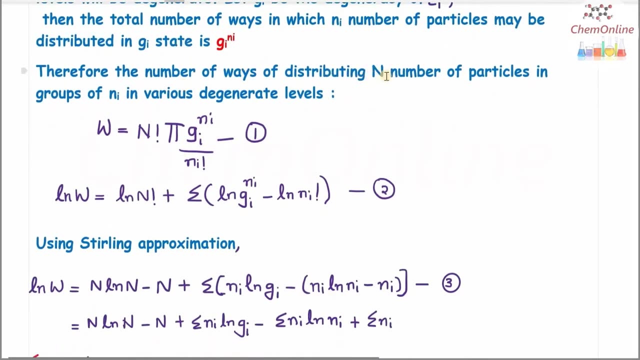 Then the total number of ways in which ni number of particles may be distributed in gi levels is gi raised to ni. Here gi is the degeneracy of the ith level and ni is the number of particles. So therefore, the number of ways of distributing n number of particles in groups of ni in various degenerate levels, 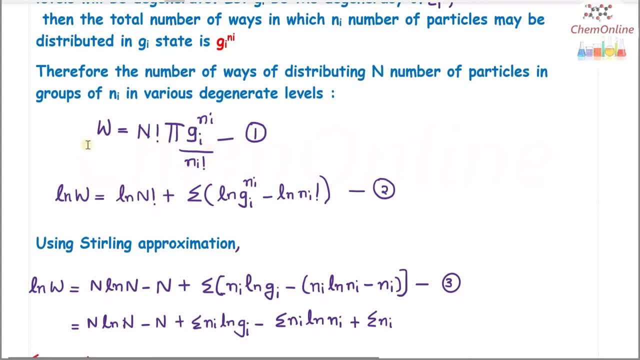 We have seen this equation earlier How different particles, identical and distinguishable particles, can be distributed in groups of ni in various degenerate levels. Here we are considering the degeneracy also, So the equation will be: w equals n. factorial into the product of gi raised to ni divided by ni factorial. 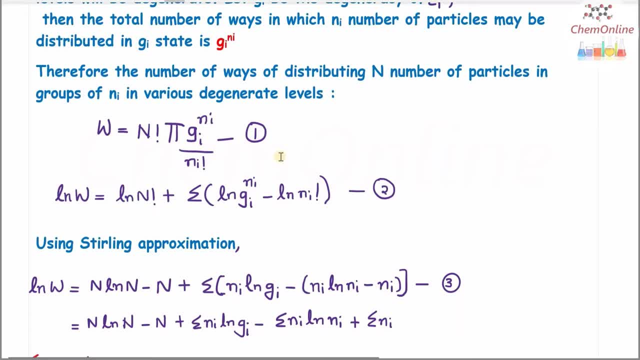 Let this be equation 1.. Now apply logarithm, So log w is equal to Log n factorial plus summation. If we give log here, log gi raised to ni minus log ni factorial. Let this be equation 2.. 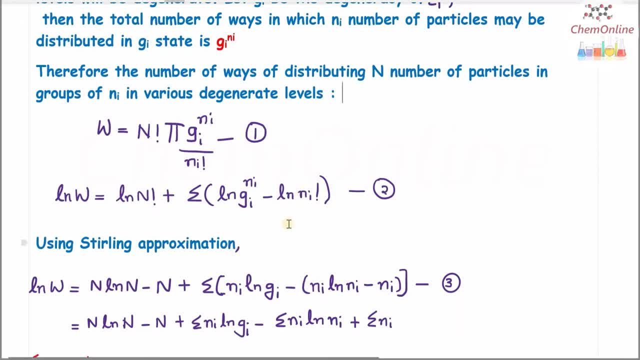 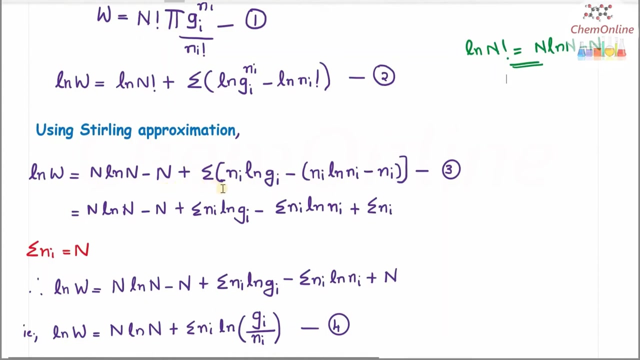 Now apply Stirling's approximation. So according to Stirling's approximation, log n factorial equals n log n minus n. So using Stirling's approximation we can write: log w equals n, log n minus n plus. summation: log gi raised to ni can be written as ni log gi minus. 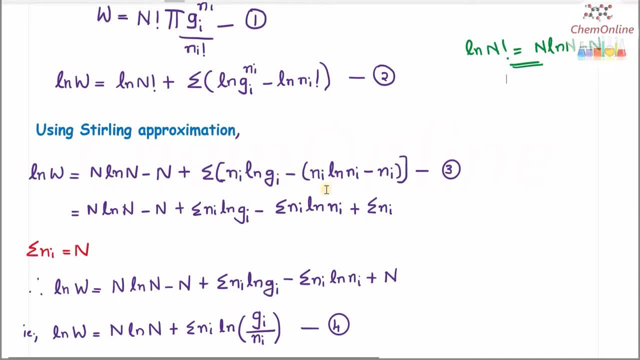 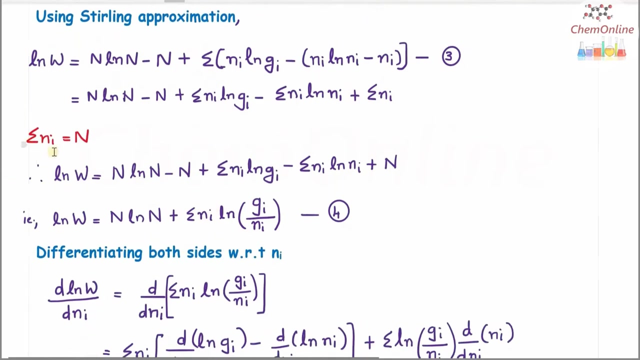 Again you have log ni factorial, So minus ni log, ni minus ni Equation 3.. Now just rearranging n log n minus n plus Summation, ni log gi minus summation, ni log ni plus summation ni. Now summation ni means it is a total number of particles which is capital N. 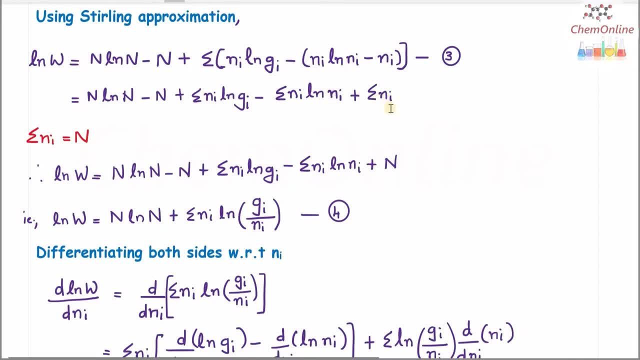 So in this equation instead of summation ni you can write capital N. Therefore log w equals n log n. minus n. plus summation ni log gi. minus summation ni log ni. So here you have minus n, and here you have plus n. 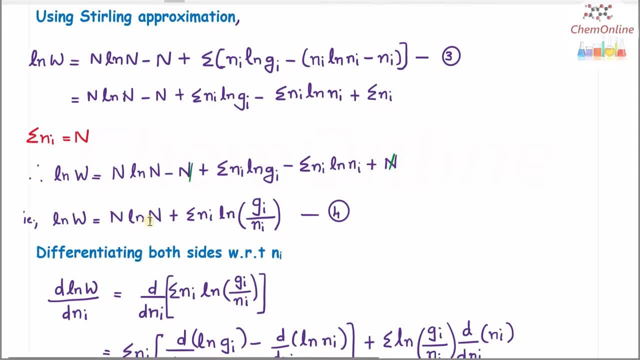 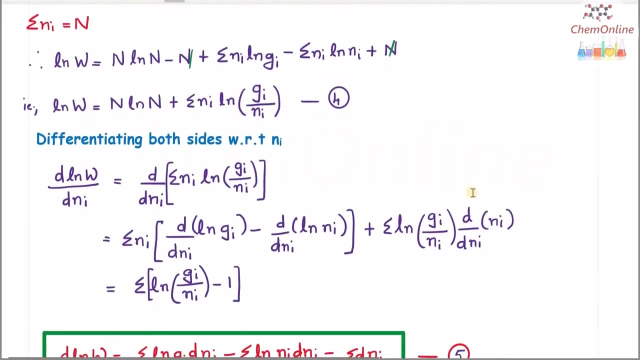 So you can write log w equals n log n plus summation ni Here log gi minus log ni So which can be written as summation ni log gi by ni Equation 4.. Now you have to differentiate both. 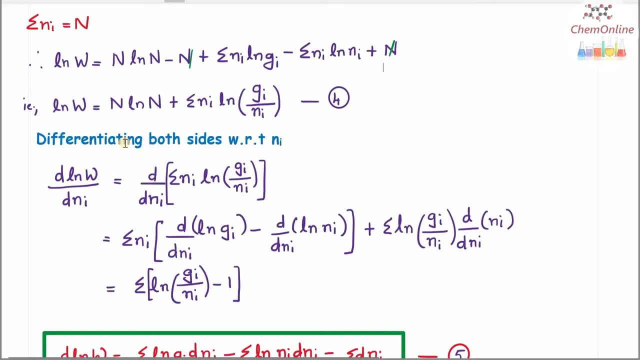 With respect to ni, That is, d log w by dni equals d by dni of summation. ni log gi by ni. See the first term. It is n log n. Capital N is a total number of particles, which is a constant, So differential of this N will be 0.. 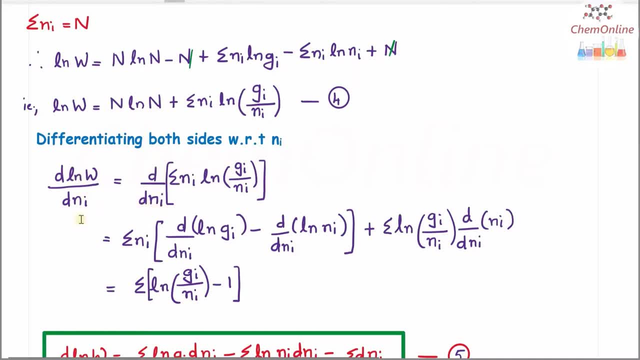 That is why we have not written the first term here. Okay, So d log w by dni, It will only be equal to d by dni of this second term. So summation ni log gi by ni So differentiate and you will get summation log gi by ni minus 1.. 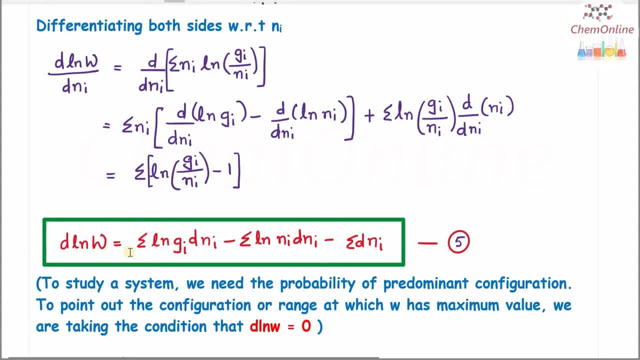 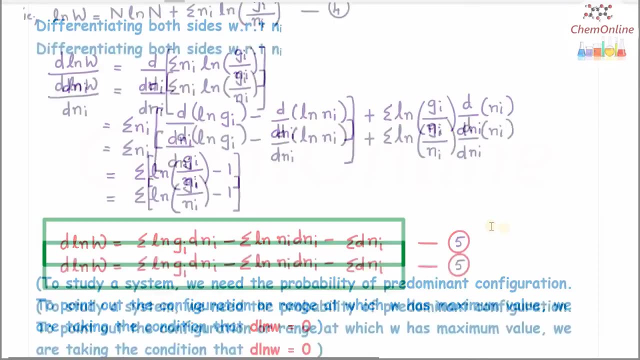 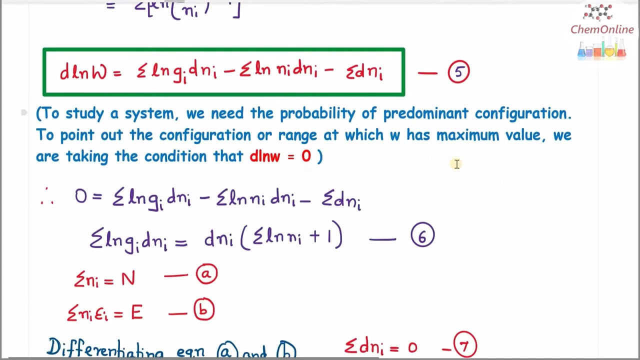 Or you can write: d log w is equal to summation log gi into dni minus summation log ni dni minus summation dni. Okay, Let this be equation 5.. Now you have to find out the probability of predominant configuration. Okay, 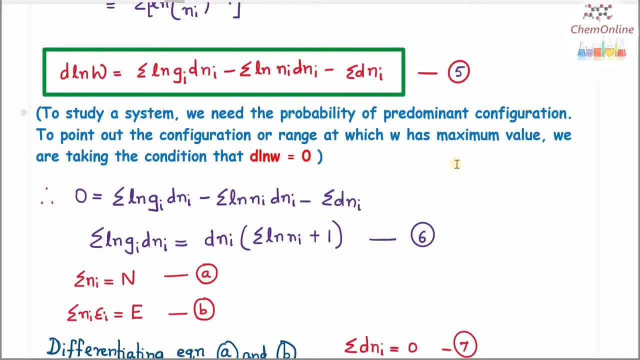 So, in order to find out which configuration will be the most probable, we have to take the condition that d log w is equal to 0. Okay, So please remember this condition, Since w denotes the thermodynamic probability. So, in order to find out the probability of the predominant configuration at which w has maximum value, 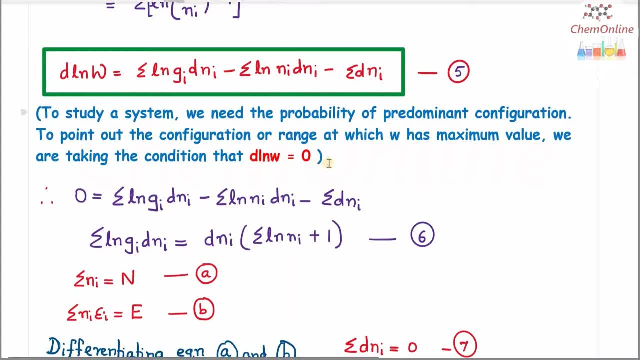 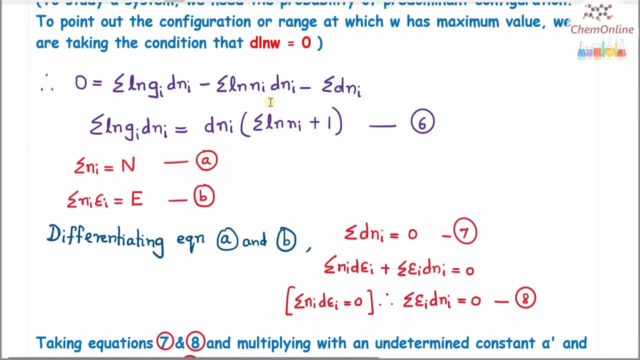 we are taking the condition that d log w equals 0. So in equation 5, put these terms: equal to 0. That is d log w equals 0. So you can write: 0 equals summation log gi dni minus summation log ni dni minus summation dni. 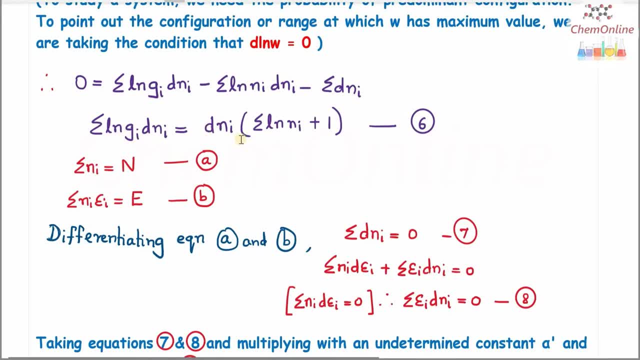 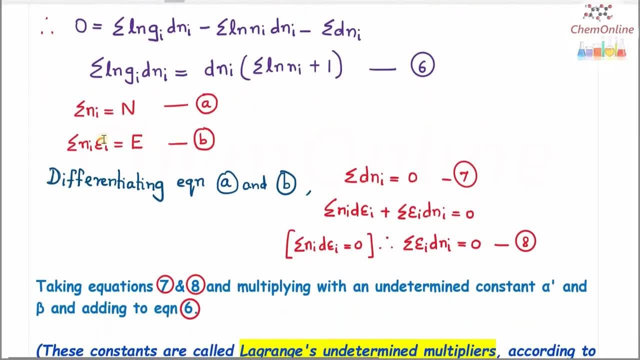 Or summation log gi dni equals dni into summation log ni plus 1. Equation 6. Now again consider summation ni equals capital N. Let this be equation A. Also summation ni epsilon i, equals capital E. 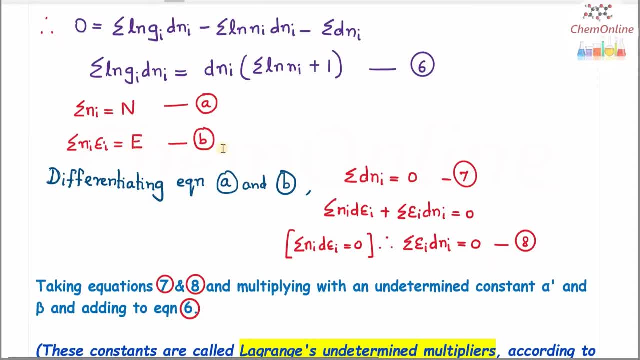 That is the total energy. Let this be equation B. Now, differentiating equation A and B, we get summation ni in a differentiator. So what do you get? Summation dni equal to 0, because summation ni is equal to capital N, which is a constant. 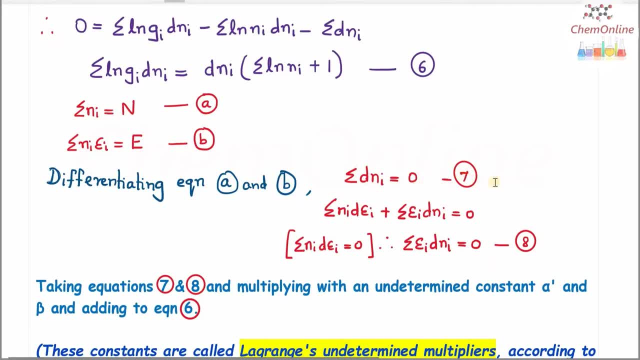 So summation dni is equal to 0.. So we have marked it as equation 7.. Okay, So summation dni equals 0, equation 7.. Now next differentiate equation B. We have summation ni. epsilon i equals E, So summation. 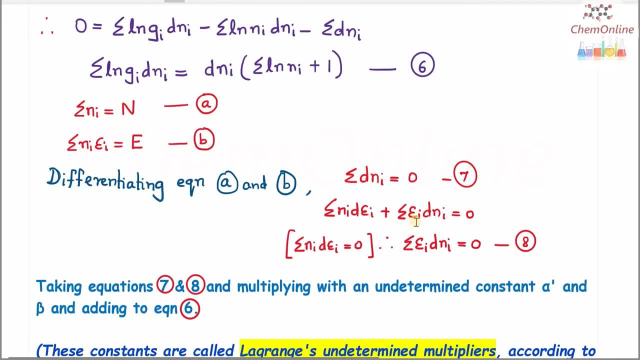 ni into d epsilon i, plus summation epsilon i into d epsilon i, Epsilon i into dni equals 0. So here summation ni d epsilon i equals 0. That means summation epsilon i dni equals 0. So you have equation 7 and 8.. 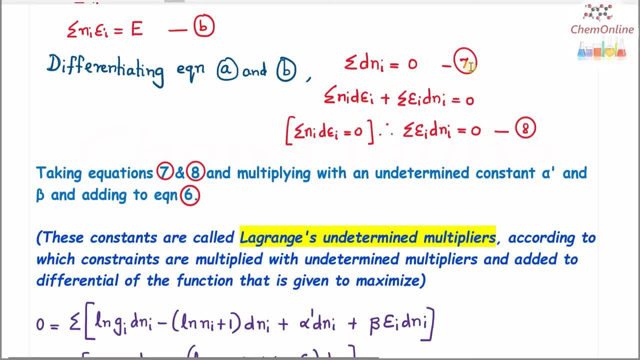 Now taking equations 7 and 8, and we have to multiply it with an undetermined constant, That is 2.. That is 2 constants: alpha, dash and beta. Multiply equation 7 with alpha and equation 8 with beta, which are 2 constants, and then 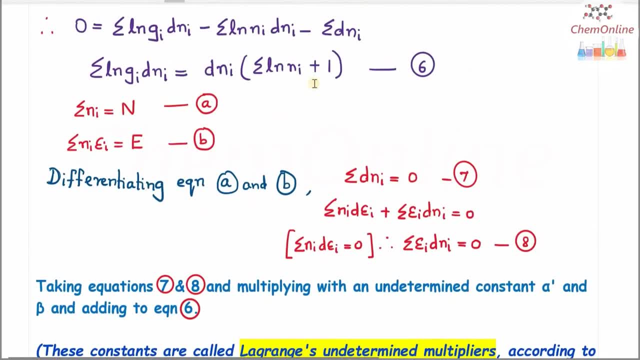 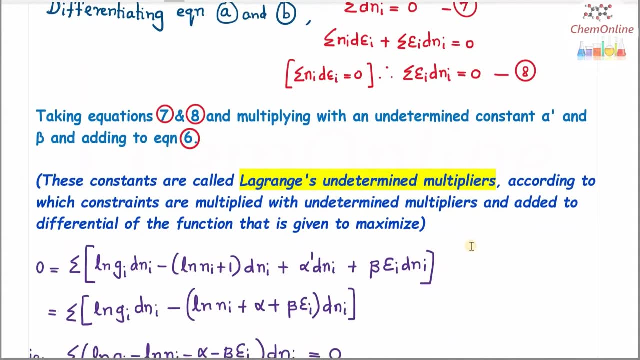 add to equation 6.. That is this equation. This is the method of Lagrange's method of multiplication. Okay, And these constants are called Lagrange's undetermined multipliers. Again, this is a method used in mathematics, So these constants are called Lagrange's undetermined multipliers, according to which 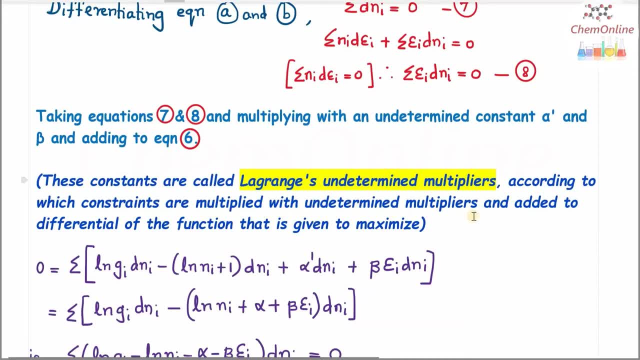 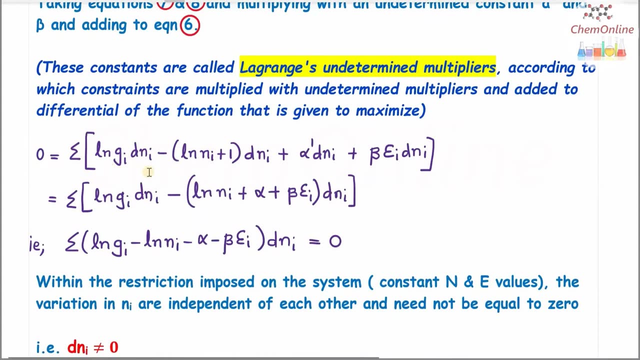 constraints are multiplied with undetermined multipliers, undetermined constants, and added to the differential of the function that is given to maximize. So accordingly you get 0 equals summation: Log gi dni minus. log ni plus 1 into dni plus equation. 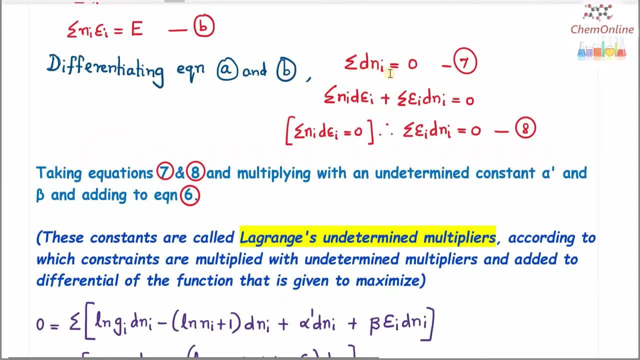 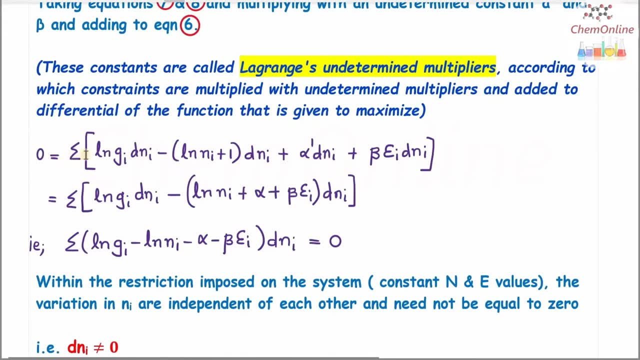 7 is summation dni, So we have to multiply it with alpha dash. So that is done here. alpha dash into dni- Summation term was commonly written outside, So alpha dash into dni plus equation: Yes, beta epsilon i dni. 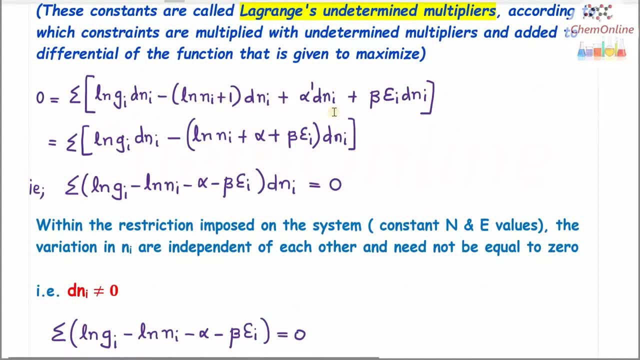 Now, dni is common, So you can den realization. I'm sorry, So you can write summation log gi dni minus. here you have log ni plus 1 plus alpha dash plus beta epsilon i, and 1 plus alpha dash is written as alpha here. 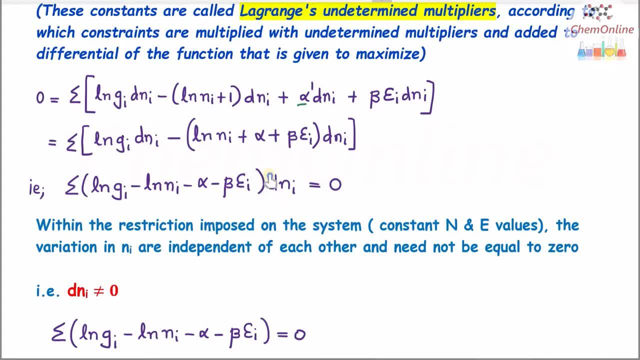 So we multiplied with a constant alpha dash, here you have 1 and alpha dash. so 1 plus alpha dash is written as alpha here. So log ni plus alpha plus beta epsilon i into dni. that is summation. log gi minus log ni minus alpha minus beta epsilon i into dni equals 0.. Now we have two terms. 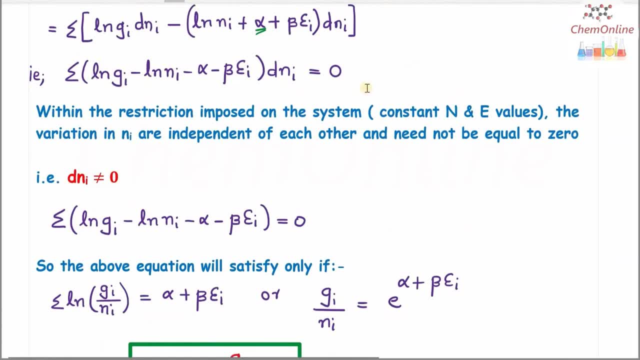 if this equation is equal to 0, either dni will be equal to 0 or this term log gi minus log ni minus alpha, dash is written as alpha here. So log ni plus alpha plus beta epsilon i into dni. alpha minus beta epsilon i will be equal to 0.. But we have a restriction on the system that 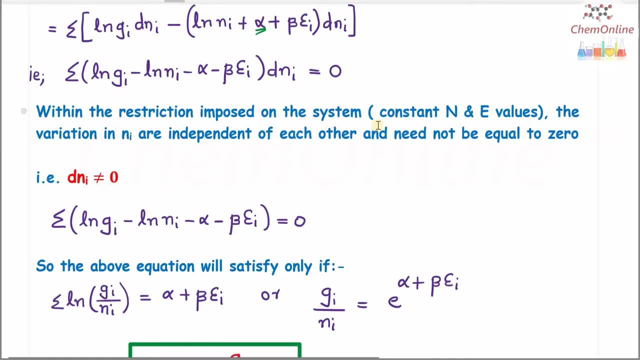 the total number of particles is a constant. the total energy is a constant. That means the variation in ni, that is, the variation of the number of particles, are independent of each other and need not be equal to 0. That means dni need not be equal to 0.. 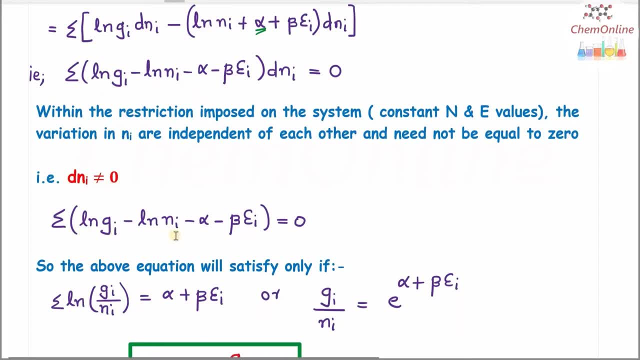 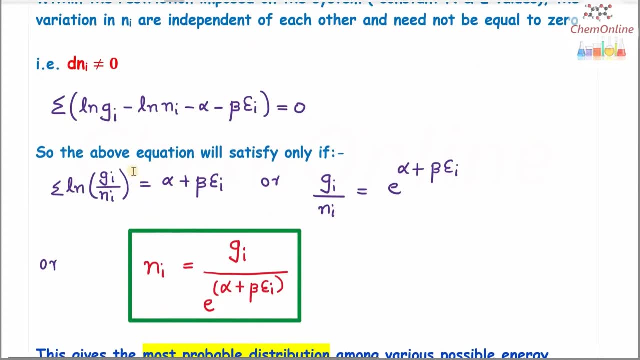 Then which term is equal to 0? So log gi minus log gi minus log ni. minus log gi minus log ni, which term will be 0. log gi minus log ni minus alpha minus beta epsilon i is equal to 0. That means summation log gi by ni equal to alpha plus beta epsilon i, or you can write gi by ni. 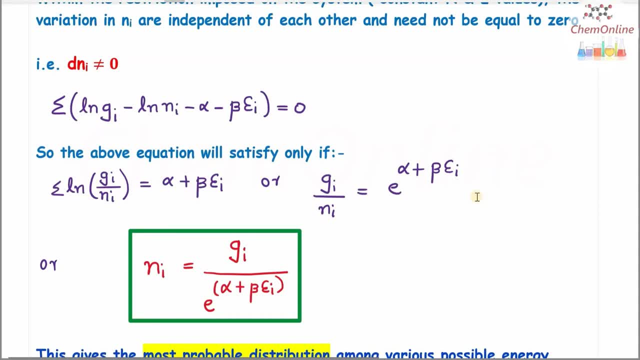 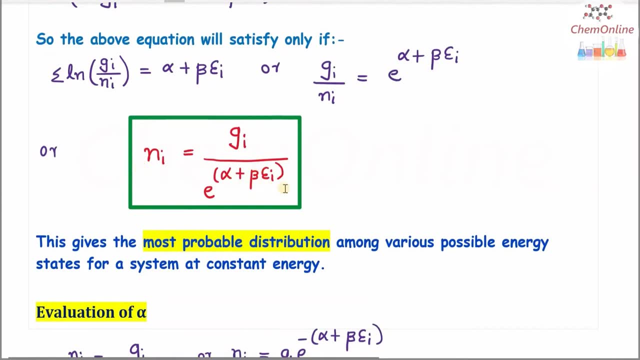 equals e raised to alpha plus beta epsilon i. or there is also another way of writing: ni equals gi by e raised to alpha plus beta epsilon i. This equation gives the most probable distribution among various possible energy states for a system at constant energy. So you have ni equals gi by e raised to alpha plus beta epsilon i. This is the 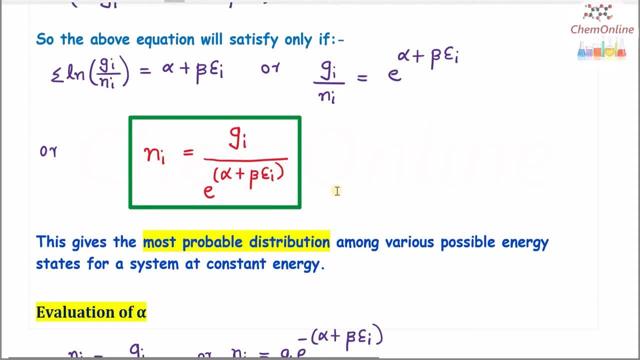 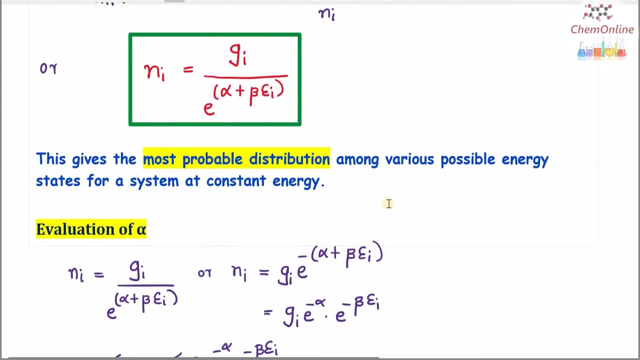 fundamental equation which represents the most probable distribution. Now you have two constants, alpha and beta. So we have to find out the value of alpha and beta, and that will complete the Maxwell-Poltzmann distribution law. Now what is ni? ni is the number of particles in each energy level, gi is the degeneracy. 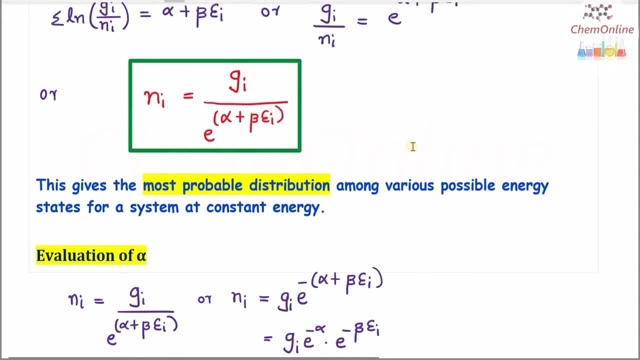 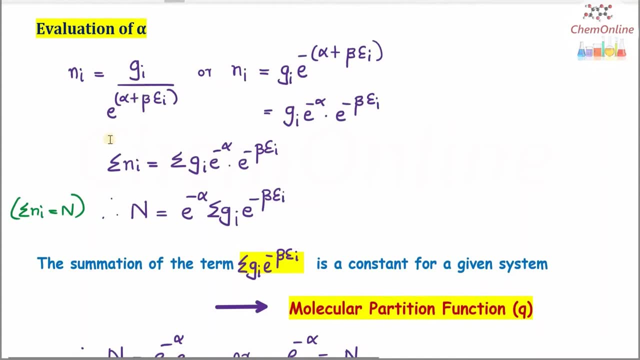 epsilon i is the energy of the ith level. Now, first we will find out what is alpha. So we have the equation ni equals gi by e raised to alpha plus beta epsilon i. or you can also write ni equals gi into e raised to minus alpha plus beta epsilon i, That is, gi into e raised to minus alpha, into e. 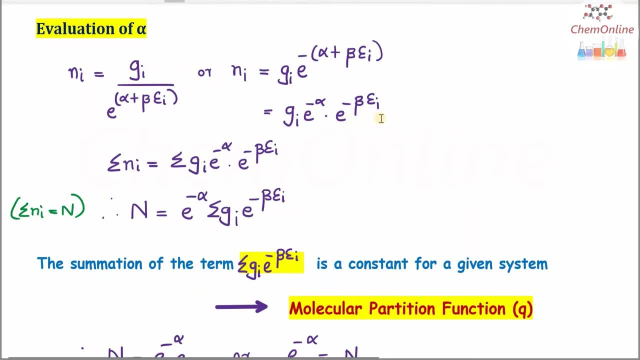 raised to minus beta epsilon. i. Now give summation to both sides So you can write: summation ni equals summation gi. e raised to minus alpha into. e raised to minus beta epsilon i. Summation ni is capital N. That is capital N. 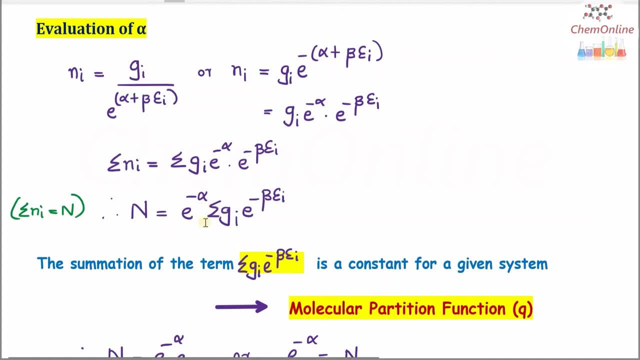 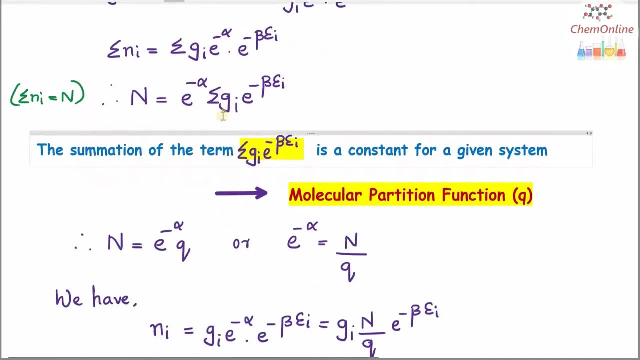 equals e raised to minus alpha, into summation gi: e raised to minus beta epsilon i. Now, this term, that is the summation of the term, summation gi: e raised to minus beta epsilon i, There is a constant for a given system which is called the molecular partition function, and this is a very important term: Molecular partition. 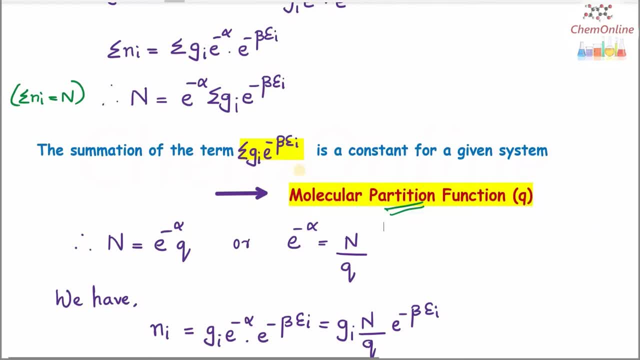 function represented as q and it is a characteristic of a system. It is a constant for a given system. Therefore, you can write: the total number of particles N is equal to e, raised to minus alpha into q. So you have written Pump On the formula that is written Prime MIC of a Process, same way that we did. 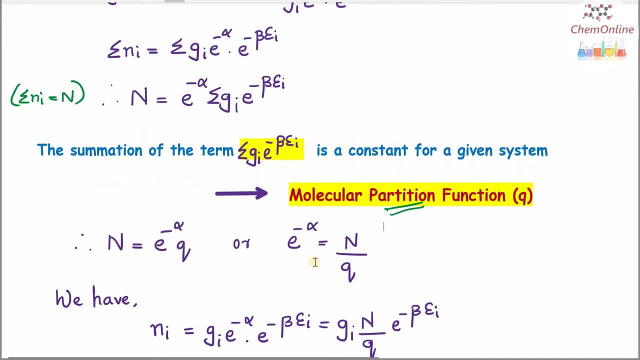 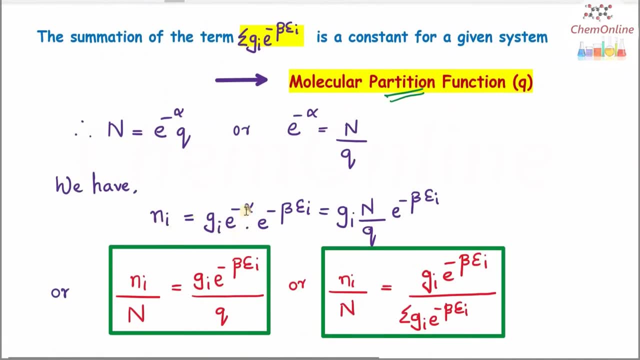 forHHH. in the previous lecture we separated from a Whoever's continuos MVM and Therefore you can write it. These are the two equations where z equals シ and 镜H equal to n by q, So you can write e price into e raised to minus alpha, into e raised to minus beta epsilon i. 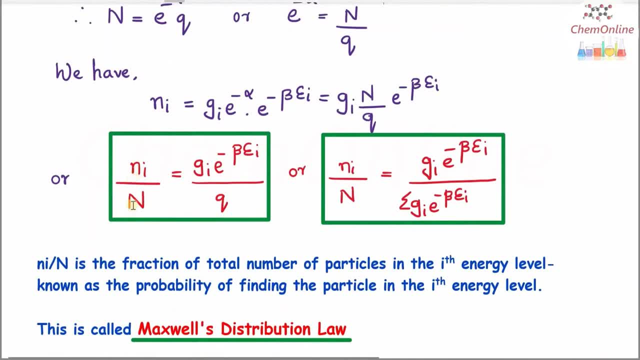 해야igh ships arts. have you noticed I justomatic new table that I have set a稿. You can write Ni by capital, N equals Gi e raised to minus beta epsilon i by Q. or Ni by N equals Gi e raised to minus beta epsilon i divided by, instead of Q. write summation: Gi e raised to minus beta. 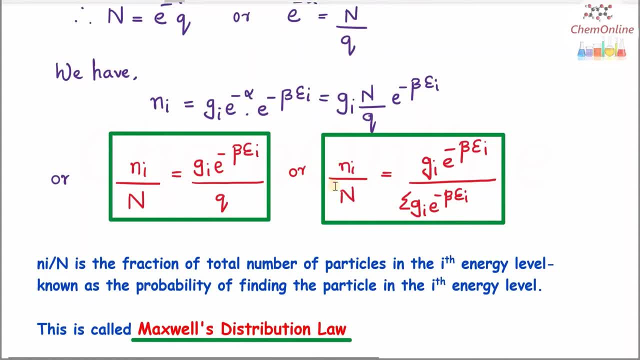 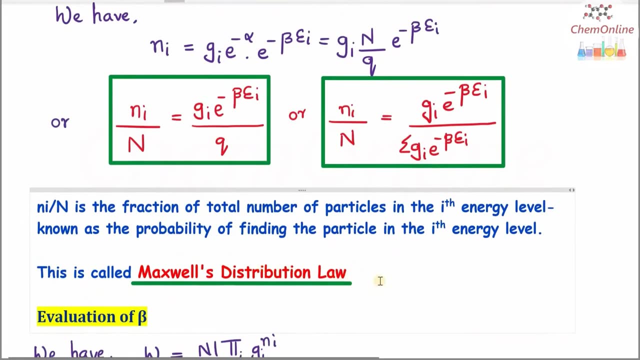 epsilon i, Ni by N, represents the fraction of the total number of particles in the ith energy level, and it is known as the probability of finding the particle in the ith energy level, and this is called Maxwell's distribution law. Now, next, you have to find out the value of beta. 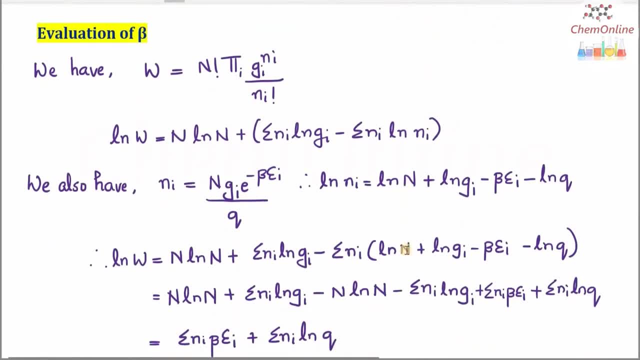 So to find out the value of beta, we are again starting from the first equation: W equals N factorial, W equals N factorial, W equals N factorial log. W equals N log N. plus summation: Ni log Gi. minus summation Ni log Ni. Now we have Ni equals capital, N Gi. e raised to minus beta: epsilon i by Q. 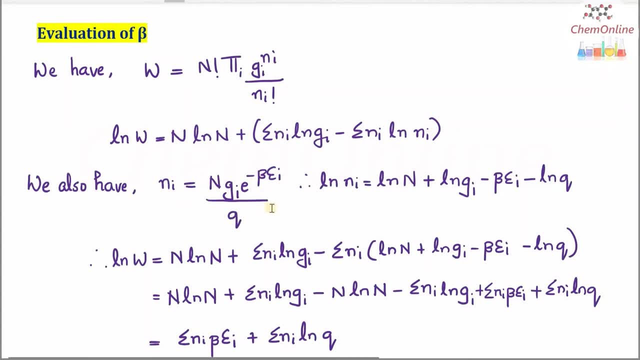 from the equation for alpha. So therefore apply log to this equation. Ni equals capital N, W equals Ni by capital N Gi e raised to minus beta epsilon i by Q. In this equation, log applies here. So you will get log Ni equals log N plus log Gi plus log e raised to minus beta epsilon i. 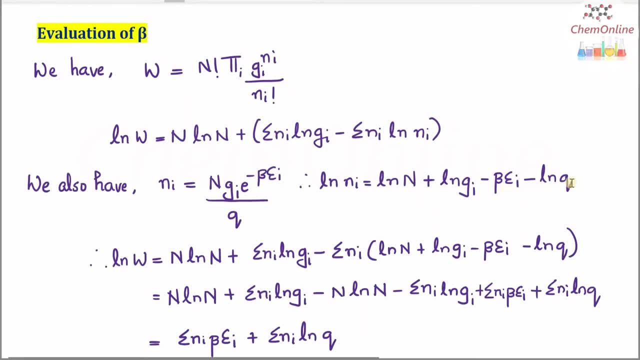 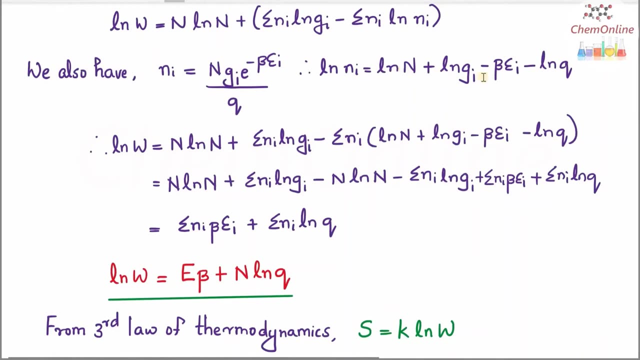 So that will be minus beta epsilon i minus log Q. Therefore log W equals N log N plus summation Ni log Gi minus summation Ni in N. So then write this So inside the bracket: log N plus log Gi minus beta epsilon i minus log Q. 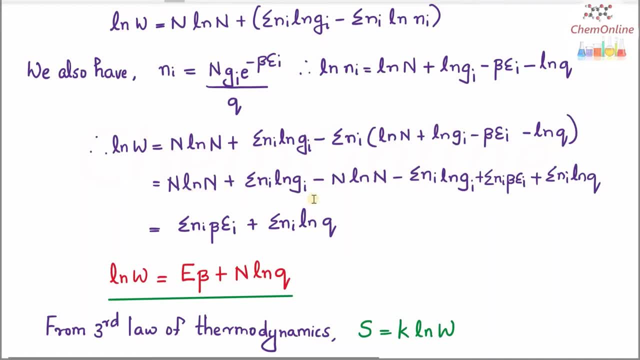 So that is N log N plus summation Ni log Gi minus. So here summation Ni log N is written as N log N minus. again summation Ni log Gi. So again summation Ni log Gi plus. summation Ni log Gi minus. summation Ni log Gi. 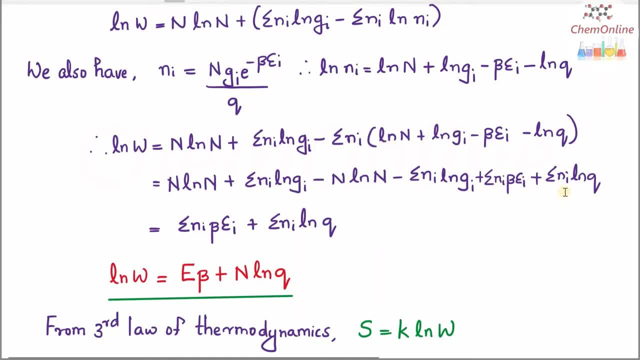 beta epsilon i plus summation ni log q. So here you have n log n minus n log n, ni log gi minus summation ni log gi. So the remaining will be these two quantities. So you can write summation ni beta epsilon i plus summation ni log q. Summation ni epsilon i is capital E. 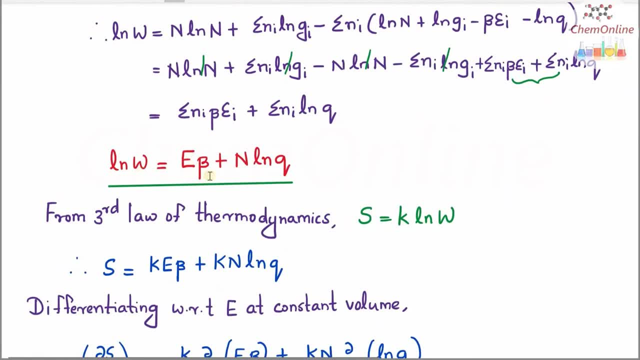 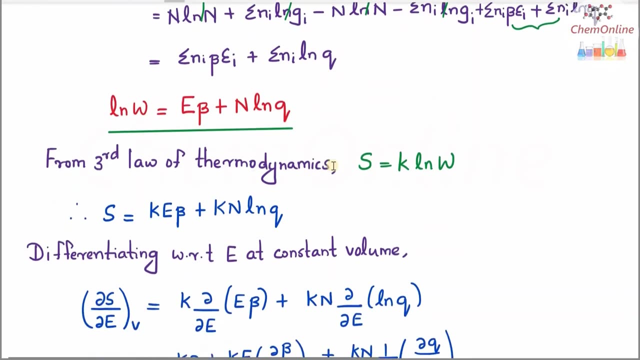 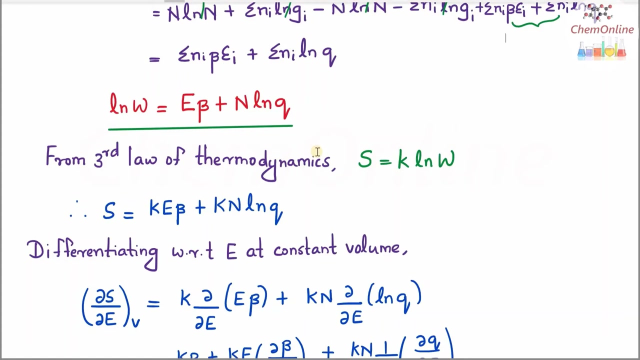 So you can write: log w equals E beta plus summation. ni is capital N, So E beta plus n log q. So you got log w equals E beta plus n log q. Now we know that the third law of thermodynamics is related to the thermodynamic probability by S. or you can say that the entropy is related to: 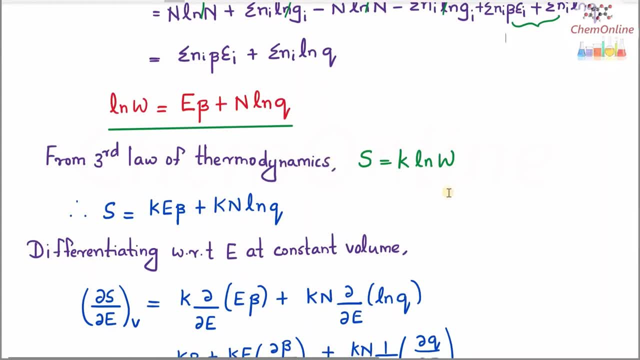 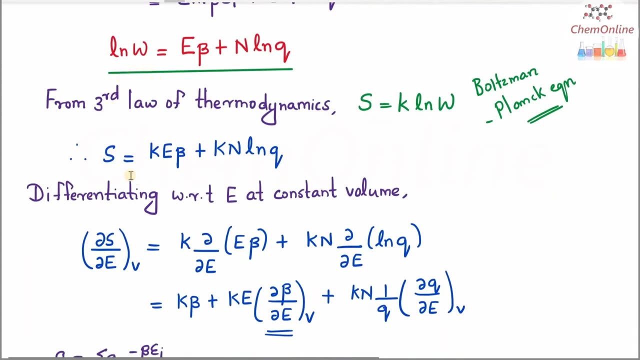 the thermodynamic probability as S. So you can write: log w equals E beta plus N log q. S equals K log w and this is also known as Boltzmann Planck equation. So we have: S is equal to K log w. Therefore S equals K into. instead of log w, substitute E beta plus N log q. 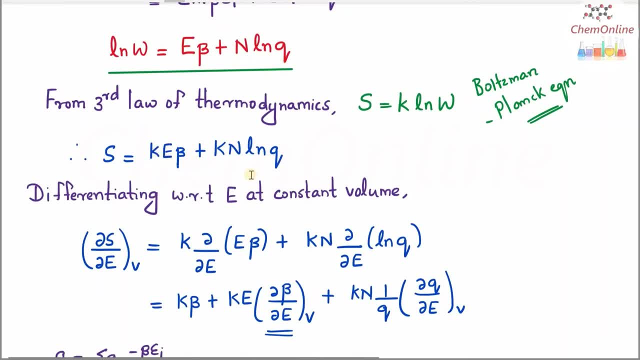 So you have K E beta plus K N log q. Now differentiate with respect to E at constant volume, That is dou S by dou E at constant v equals K into dou by dou E of E beta plus K N into dou by dou E of log q. Here K and N are constants, So K into dou by dou E of E beta. 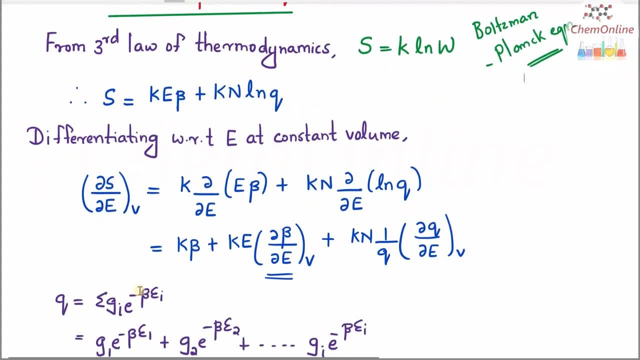 plus K N into dou by dou E of log q, Which is equal to K beta plus K E into dou beta by dou E at constant v plus kn into dou by dou u of log q will be 1 by q dou q by dou e at constant v. 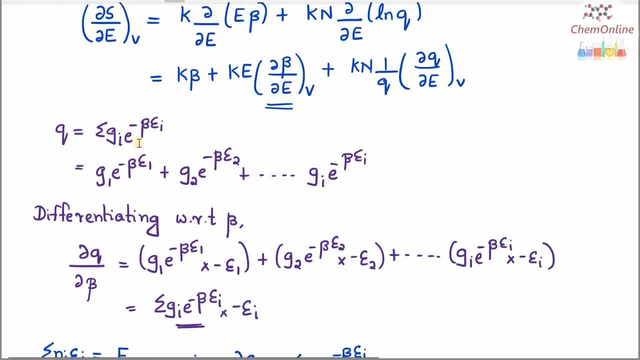 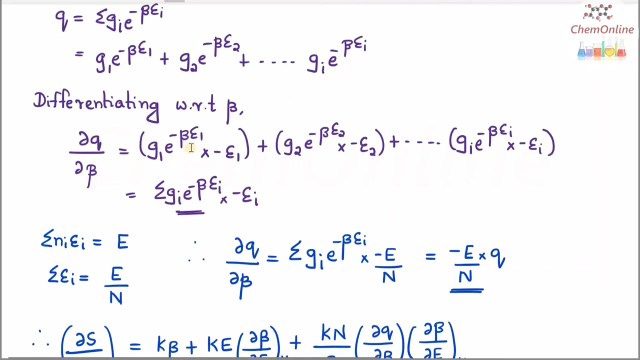 Now the partition function q equals summation gi. e raised to minus beta epsilon i, which is equal to g1. e raised to minus beta epsilon 1 plus g2. e raised to minus beta epsilon 2 plus, etc. Differentiating this with respect to beta, we will get dou q by dou beta equals g1 e raised. 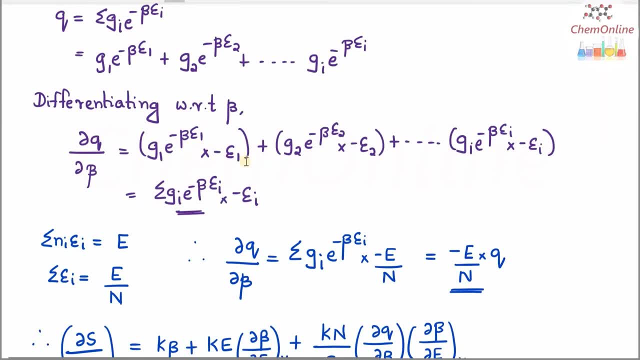 to minus beta epsilon 1 into minus epsilon 1 plus g2 e raised to minus beta epsilon 2 into minus epsilon 2 plus etc. So we can write: dou q by dou beta equals summation gi e raised to minus beta epsilon i into dou q by dou beta. 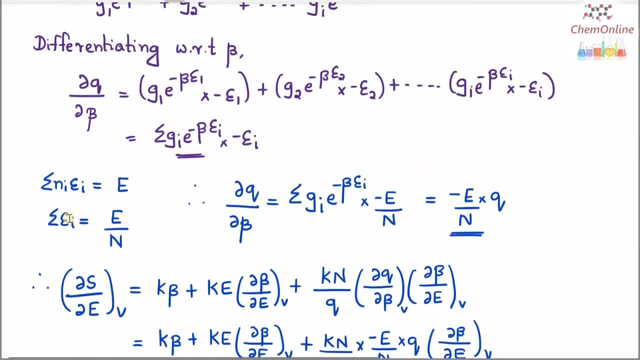 Again we have summation ni epsilon i equals e or summation epsilon i will be equal to e by summation ni, that is, e by capital n. So you can write dou q by dou beta equals summation gi. e raised to minus beta epsilon i into. instead of summation epsilon i you can write minus e by n. 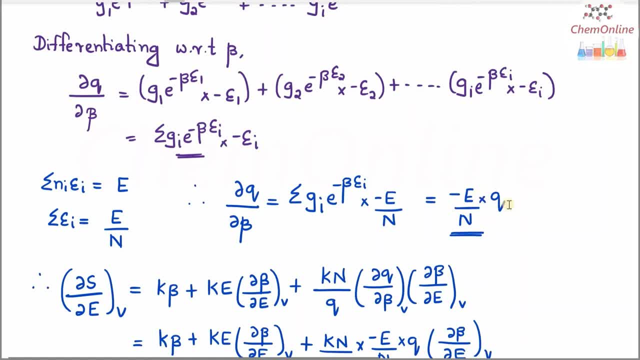 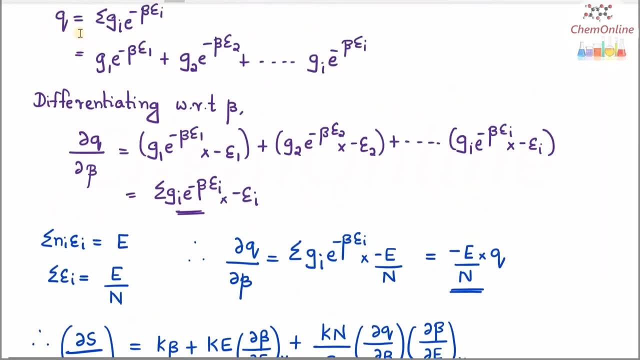 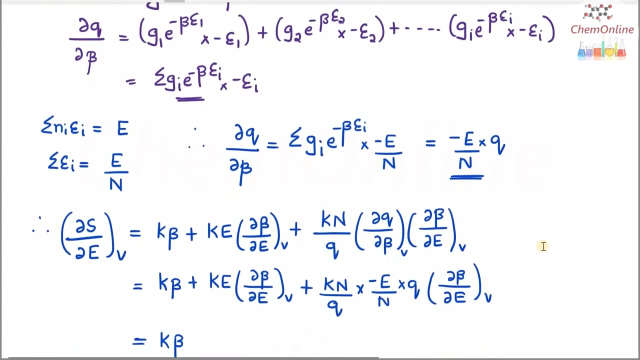 So that is equal to minus e by n into q. So please remember, we have written the molecular partition function which is differentiated with respect to beta, and you will get in this form Now summation: epsilon i is written as e by n, So dou q by dou beta will be minus e by n into q. Now, substituting in dou s by dou e at constant v: 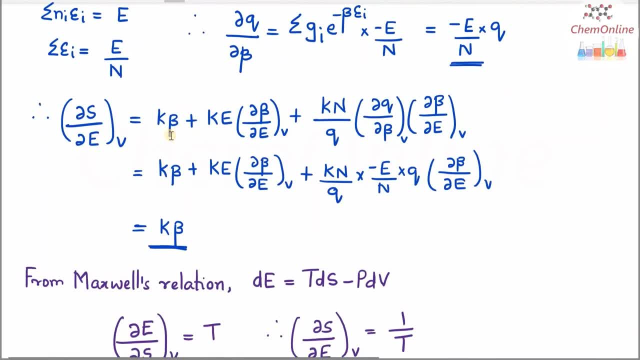 So dou s by dou e at constant v will be equal to k beta plus ke into dou beta by dou e at constant v plus kn by q, into we have dou q by dou e, which is written as dou q by dou beta at constant v into dou beta by dou e at constant v. Now here substitute for dou q by dou beta, which is minus. 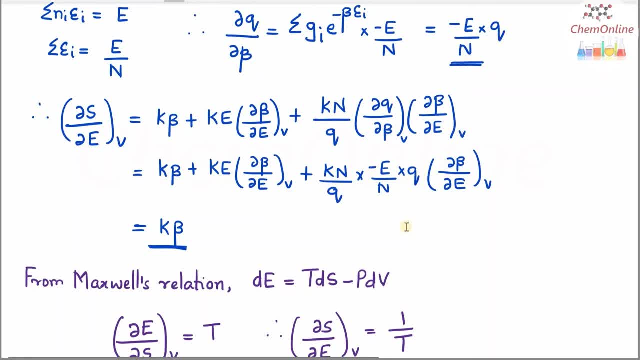 e by n into q, So that is written here. So we have ke into dou beta by dou e here. Here also: n and n will get cancelled, q and q will get cancelled. So here minus ke dou beta by dou e, So the remaining will be k beta. So you got dou s by 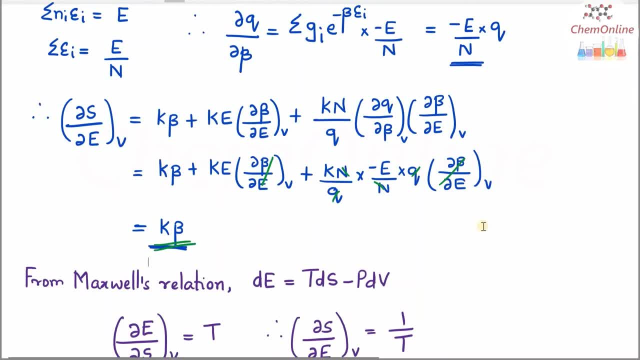 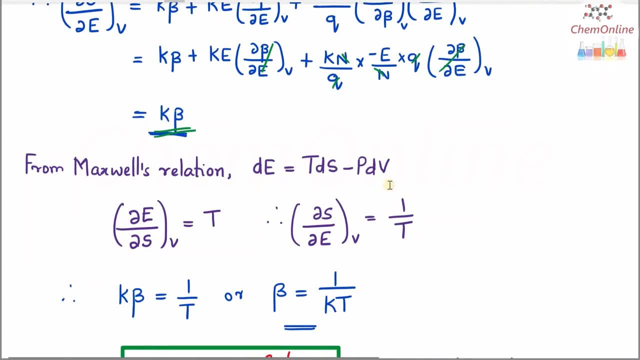 dou e at constant v equals k beta. Now again from thermodynamics, we have the Maxwell's relation: d e equals p d s minus p d s. So we have dou e by dou e at constant v equals k beta. If the volume is constant, d v equals zero. This term will not be there, only t d s. So you can write. 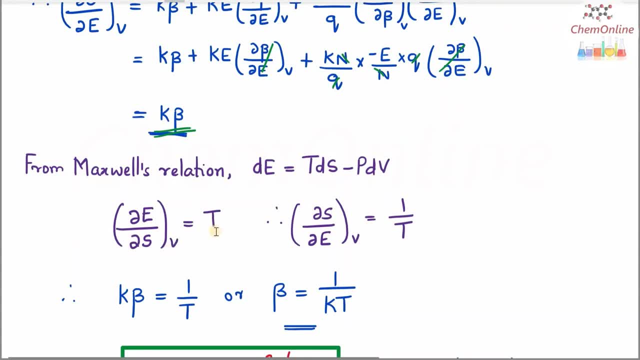 dou e by dou s at constant v equals t. Therefore dou s by dou e at constant v equals 1 by t. Here we have dou s by dou e at constant v equals k beta. From the Maxwell's relation we get dou s by dou e at constant v equals k beta. So we have dou e by dou e at constant v equals k beta. 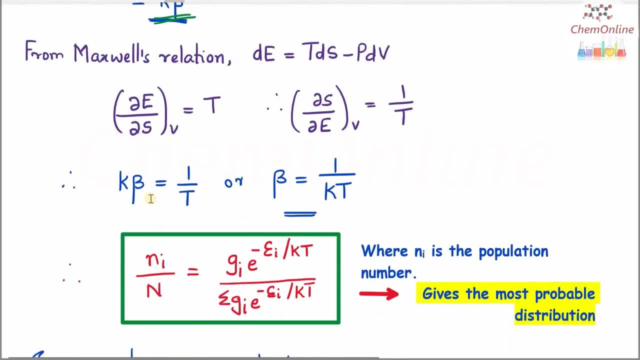 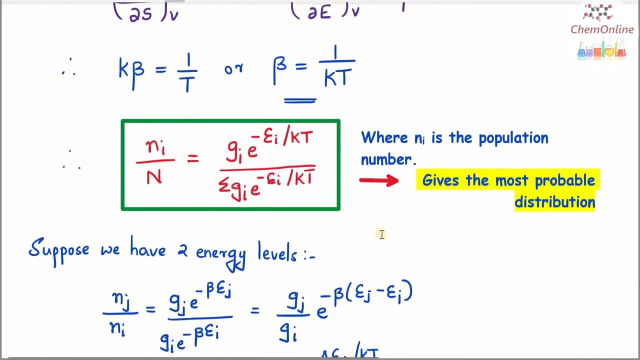 So we have dou e by dou e at constant, v equals 1 by t, That is, k beta equals 1 by t or beta equals 1 by kt. So we have got the value for beta, which is equal to 1 by kt. Therefore, we can modify the. 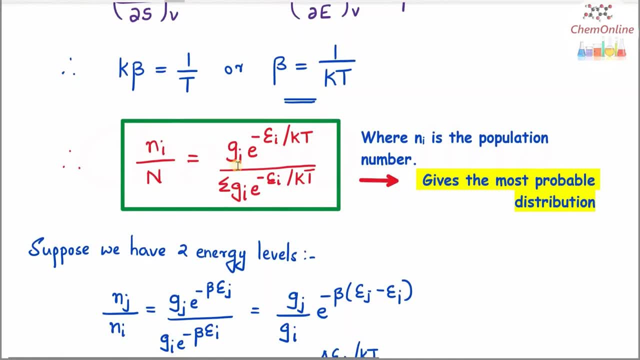 Maxwell's relation. as n i by n equals g, i e raised to minus. We had beta epsilon i instead of beta right, 1 by kt. So e raised to minus 1 by kt. So we have dou e by dou e at constant v equals 1 by t. 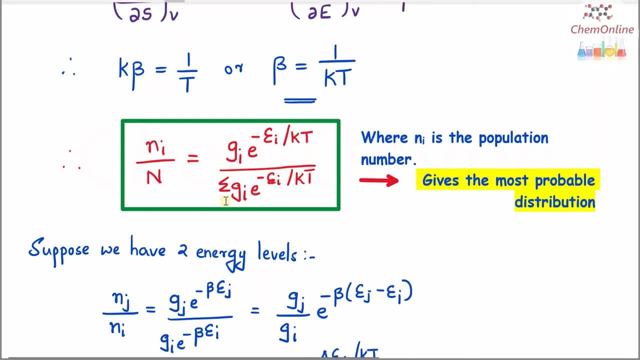 So we have dou e by dou e, raised to minus epsilon i by kt, divided by summation g i e raised to minus epsilon i by kt. Here n, i is the population number, and this equation gives the most probable distribution. T is the temperature and k is the Boltzmann constant. Now suppose we have two. 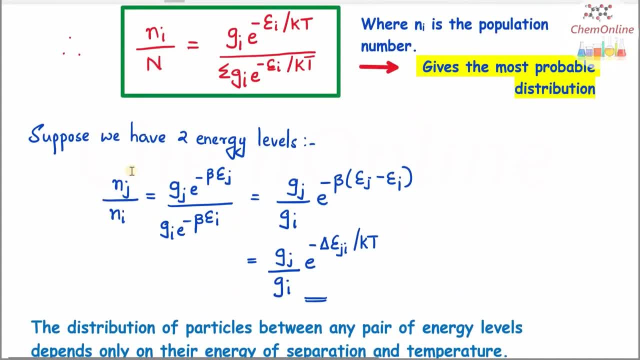 energy levels: magician epsilon g and epsilon i. So the number of particles in this level, If we take the ratio, We may have 2 energy levels. So the number of particles in this level, If we take the ratio n? j by n? i will be equal to g, j e raised to minus beta. epsilon j divided by g? i. 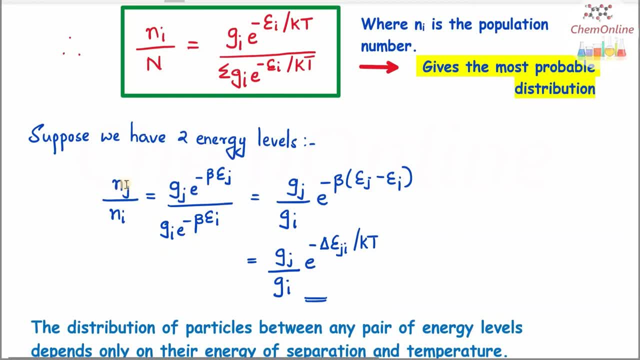 e raised to minus beta. epsilon i. Each of these case denominator is the partition function, which is a constant. So we have written only these, these two terms, only then numerator terms. So we have n. j by n. i equals g, j. e raised to minus beta. epsilon j divided by g. i e raised to minus beta. 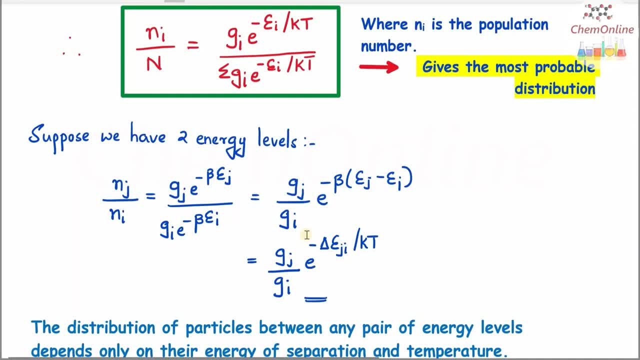 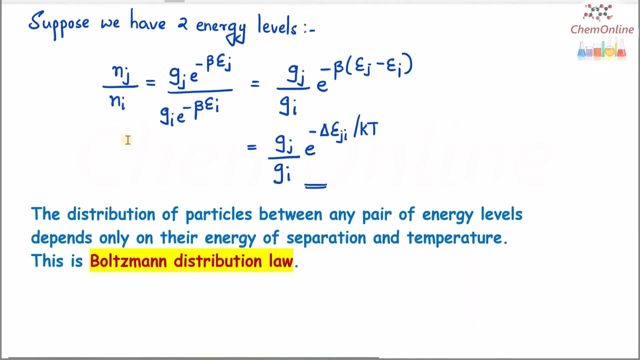 epsilon i, That is equal to g j by g i e raised to minus beta. epsilon j minus epsilon i, which can also be written as g j by g i into e raised to minus delta. epsilon j i divided by kt. So from this we can say that the distribution of particles between any pair of energy levels 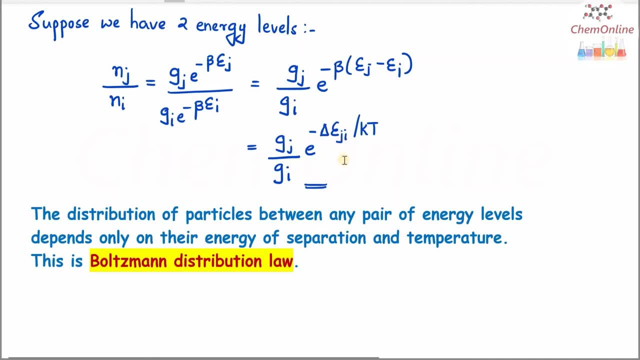 will depend only on their energy of separation, That is, delta epsilon and also temperature, Since n j by n i equals e raised to minus delta epsilon by kt. So the distribution of particles between any two energy levels will depend only on the energy of separation and temperature, and this is known as Boltzmann distribution law.